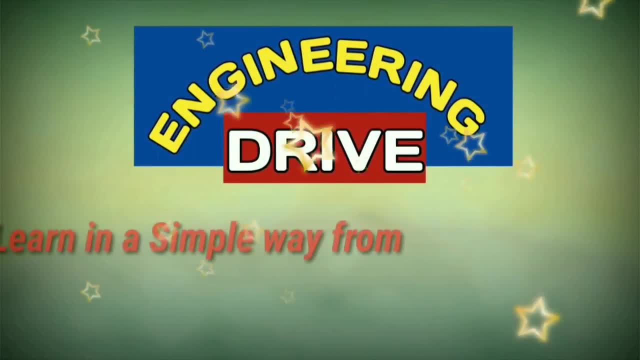 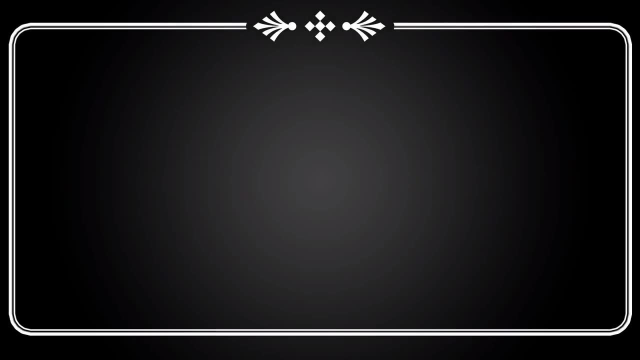 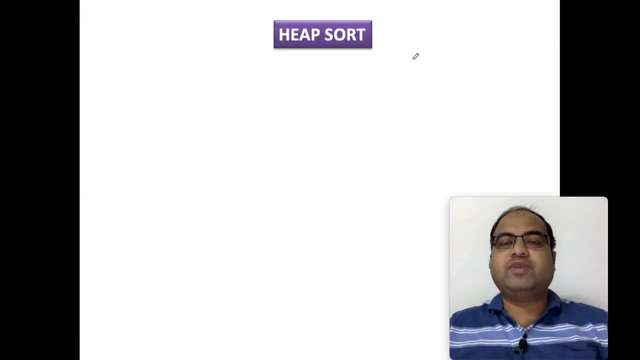 Hi, everybody, hope you are all fine. This is Atik. Welcome to our YouTube channel, Engineering Drive. Let us now discuss the working of heap sort in my today's class. So, dear students, this heap sort or the heap techniques are very, very important concept in data structures. and question may ask. 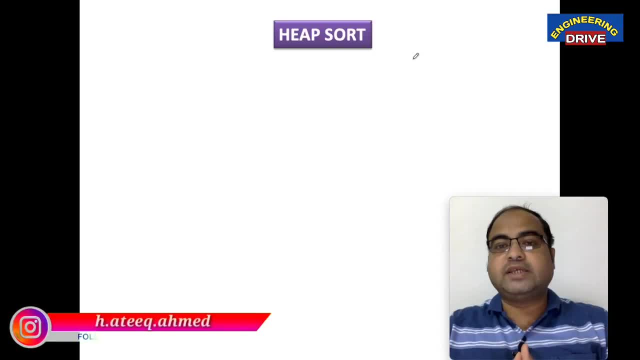 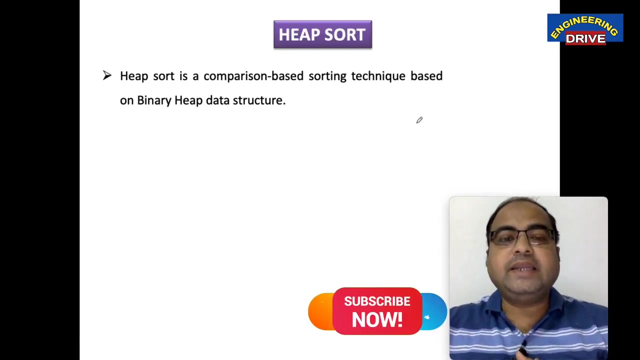 in any way. So what are the types of questions also you may get in exam? I am going to discuss that also in my today's class. So without wasting the time, let us start our today's session. So point number one: heap sort is a comparison based sorting technique based on binary heap. 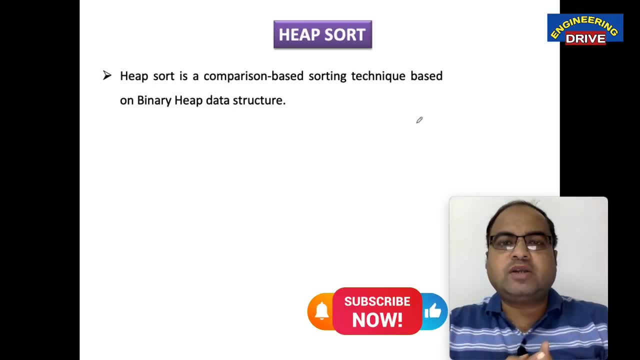 data structure. Now, there is one unique thing in heap sort. Unlike other sorting methods which I have completed, this heap sort relies on binary tree concept. So what is the binary tree? Already, we know that I have prepared several videos on different concepts of binary trees. You can go. 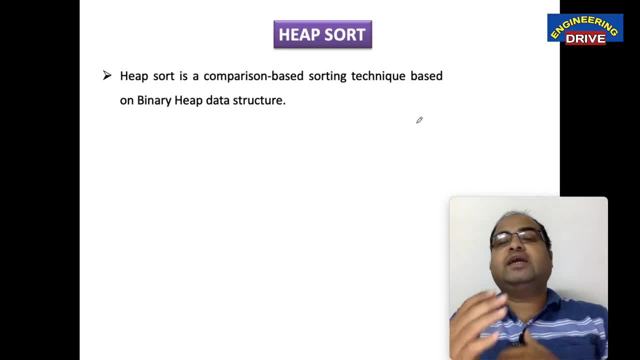 ahead and watch that in our data structures playlist. Okay, heap sort also relies on binary tree concept. How it will make use of binary trees also, you will come to know. Okay, next thing: it is similar to selection sort, where we first find the minimum element and place the minimum. 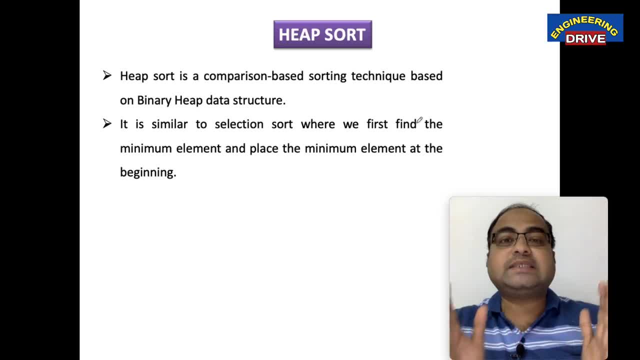 element. So heap sort is a method which will work for ascending order. Dear students, sorting doesn't mean only we need to generate the data in ascending order. Even descending order is also one type of sorting. But generally in exam, if they won't mention any ascending order or descending, 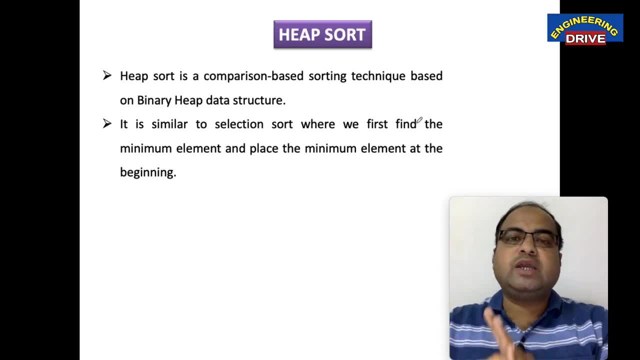 order. simply, if they ask you sort the following list of numbers, then by default, you need to sort in ascending order only. It is recommended. Okay, now, in order to generate an ascending order, what we need to do is we need to sort the data in ascending order. So what we need to do is: 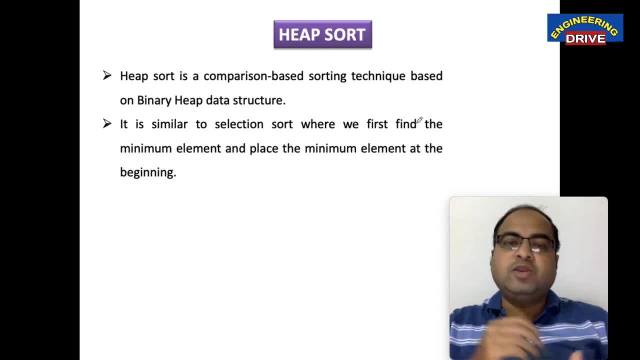 minimum element. we need to keep at the beginning. in order to generate a descending order. we need to keep the maximum element at the beginning. okay, next point: a binary heap is a complete binary tree, because here we are going to generate one heap that is a binary heap. now, a binary heap is a. 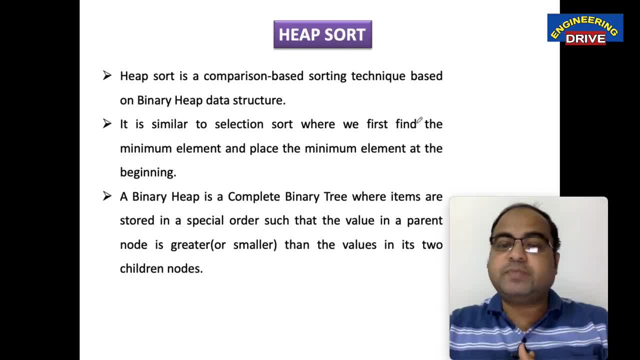 complete binary tree where items are stored in a special order such that the value in a parent node is greater or smaller. see the important point here: greater or smaller. we are not using only greater word here. even it can be greater or smaller than the values in its two children. 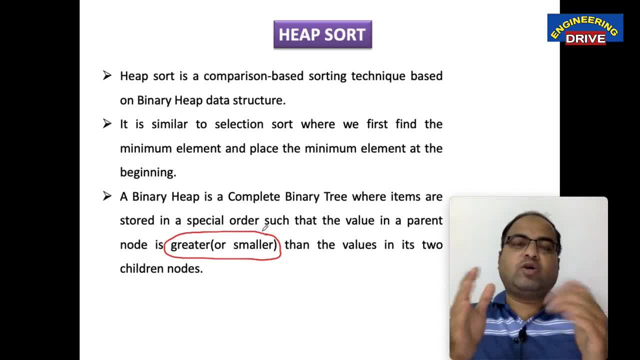 nodes or child nodes. now here the concept of heap is: whenever we are generating a heap, there is one terminology we need to follow. first point: a heap is a binary tree. so in we know that in binary tree every node will have maximum number of nodes and every node will have maximum 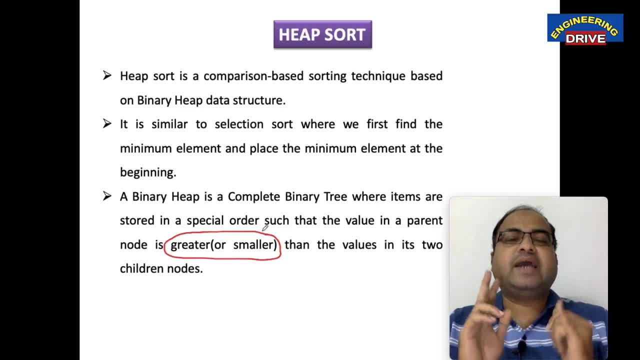 two child nodes, not more than that maximum two. it can have one, or it can have maximum two child nodes, which is a binary tree concept. now in heap, there is one condition. what is that condition? the parent node value must be greater than the child nodes. that is one case, or the parent node 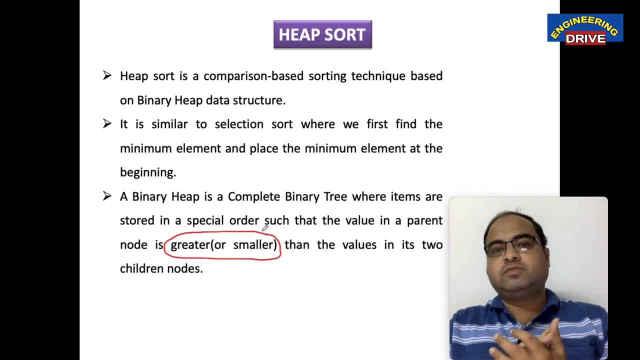 or root node value must be less than the child nodes. these are the two types of heaps we will discuss in our heap sort method. okay, next point. a binary tree is a binary tree, which is a binary warnthe former is called max heap and the latter is called mean heap. so in max heap the parent node, 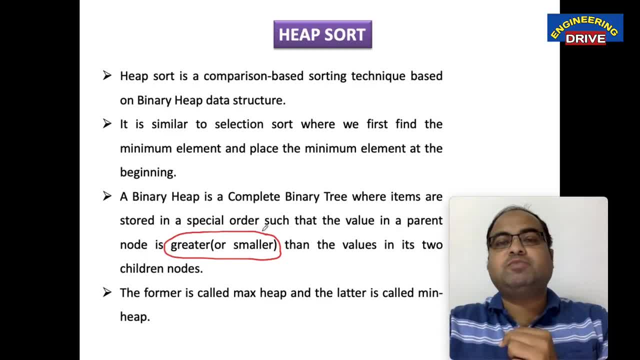 value will be greater than the child nodes. in mean heap, the parent node value will be smaller the child nodes. you remember this one, okay? the heap can be represented by a binary tree or array. so this heap can be generated, represented either by using binary tree or we can make use of array also. 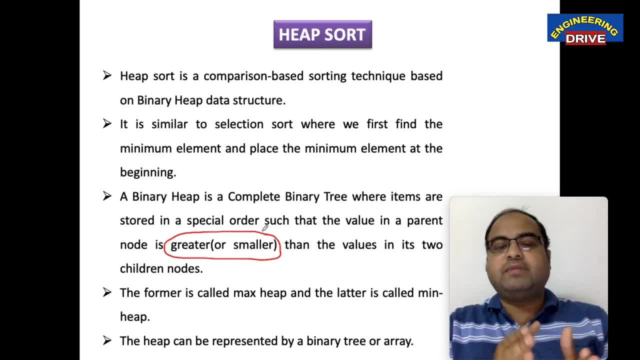 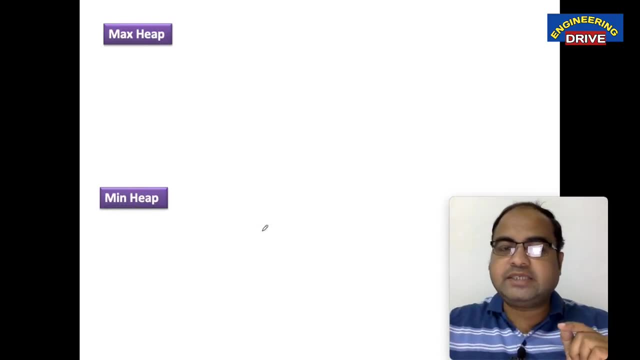 but non-linear data structures. so this heap can be represented by using either of these two methods. but in my today's video i will be showing you the first method: how a heap can be generated by using a binary tree now. so now there are two types of heaps. i told you max heap and min heap, so let me 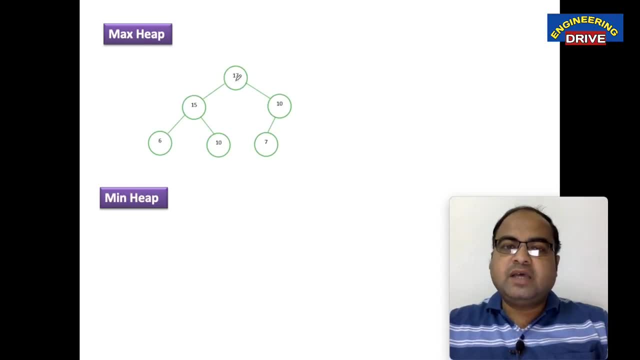 show you the difference between them. you can see here in max heap the root node value is 17, whereas its child nodes values 15 and 10. so root node value is greater than the child nodes. similarly you can see this one: 15 value is greater than 6 and 10 child nodes. 10 value is greater than the. 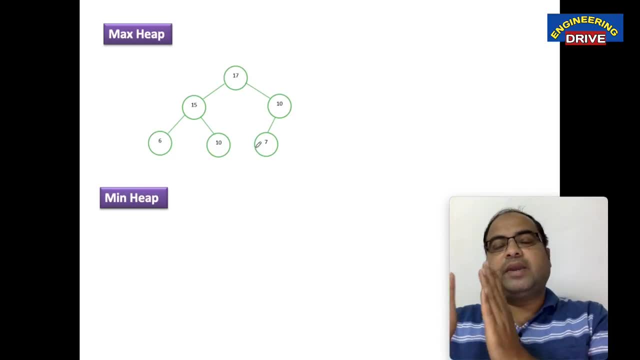 child node 7. this is a max heap. in max heap the parent value will always be greater than their child nodes or children nodes. you remember this point? what happened in min heap? opposite the parent or root node value will be smaller than the child nodes. opposite of max heap is min heap. now in exam you may get questions in different ways. construct a. 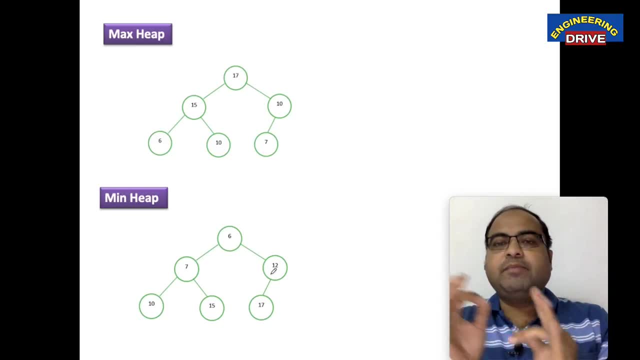 max heap from the following list of numbers: or construct a min heap from the following list of numbers, or construct a heap from the following list of numbers. if they ask you, then you can give both examples of max heap and minimum heap, depending on the marks of the questions: how. 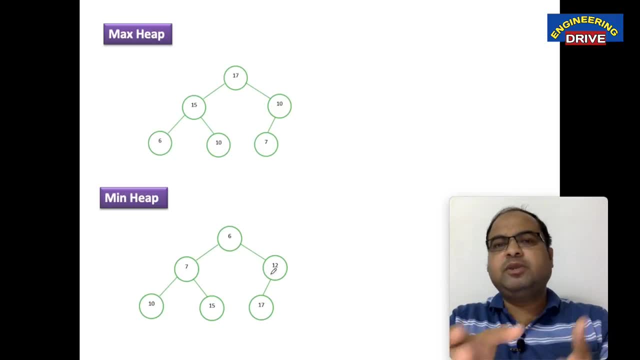 many marks if the question is asked only for five marks, simply you can write for max heap. it is more than enough. now, in my today's class, i will show you practically now, because practical example is important for us. theoretically explain to you now. let me give an example and let me show you how to generate a heap. now question: construct a. 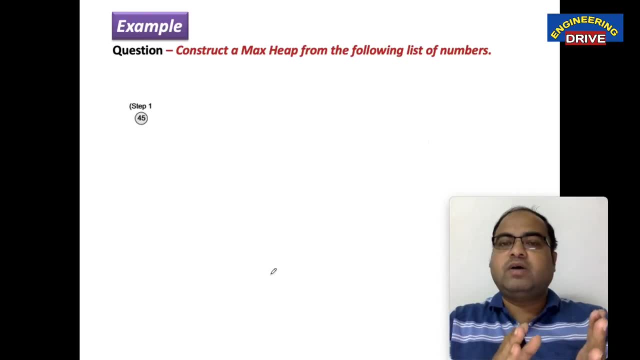 max heap from the following list of numbers. now i am going to generate a max heap now in max heap, whether root node contains maximum value or minimum value in max heap always the root node or parent node contains the max heap. so i will show you practically now, because practical example is. 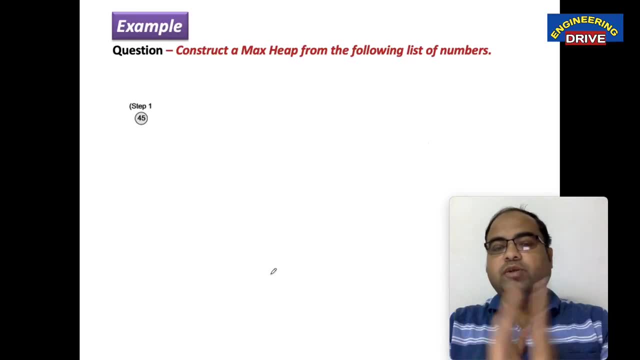 the maximum value or largest value. you remember this point. now, this is the set of numbers i have taken in this example: 45, 36, 54, 27, 63, 72, 61, 18- and by using these numbers, i am going to generate a max. 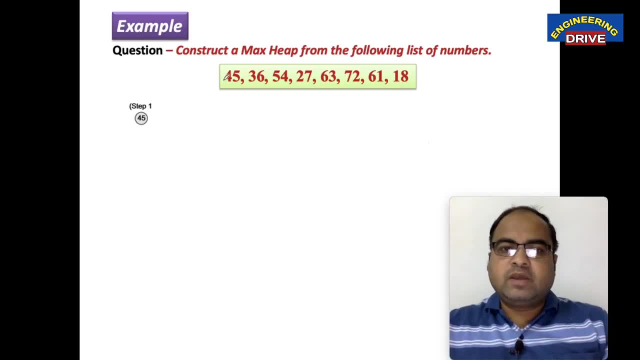 heap now. okay, so first step: take the first number in the array, whether it is sorted or unsorted, you leave that. take the first element and mark it as a root node. that's what you need to do. so which here now? first element: here we have, we have 45. so 45 i have taken and i have kept it as a root node. 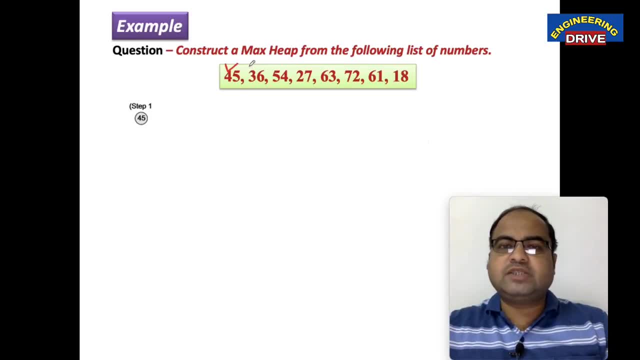 that is step number one. now, which is the next element in my list of array? in this array i am having the next element, 36. so take 36 and where we need to keep the 36 you know as a left child of this root node, see here: left child of 45, 36. now take the third number. what is the third number? 54. 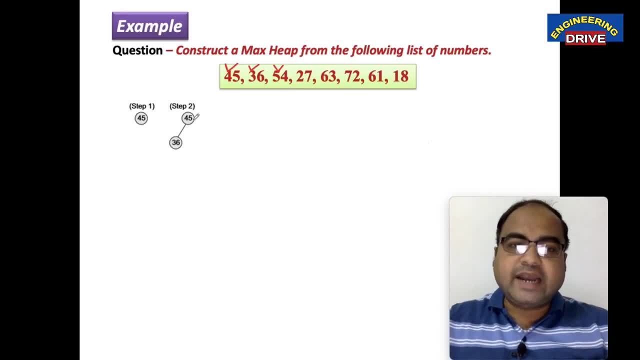 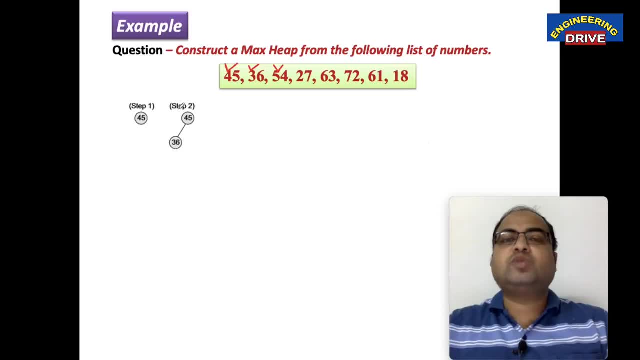 need to check, you know, the top value. always it should remain higher. the parent value should be greater than the child nodes, because that is the condition of max heap that we need to keep in brain, keep in our mind. okay, 45 is greater than 36, no problem, so insert this 54 here. 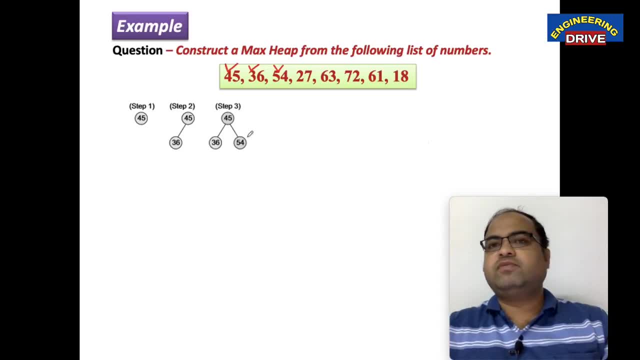 we should insert this 54 here at the right side of 45. now we can see that it is not following the max hip condition because parent node or root node is smaller than the child node, which doesn't want in max hip. that's why what we need to do, we need to swap them. so swapping will occur here, so 54 will. 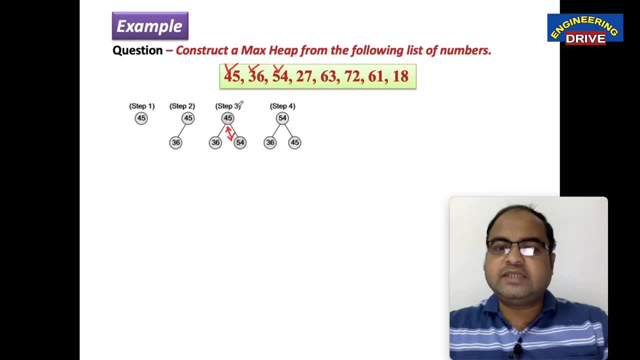 come to the root node or parent node position now. whether it is satisfying max hip condition, yes, no problem. now. next, select the next fourth element to be inserted. you know where we should insert this element, always and now. this binary tree has been completed. now now, below 36, it will become the left. 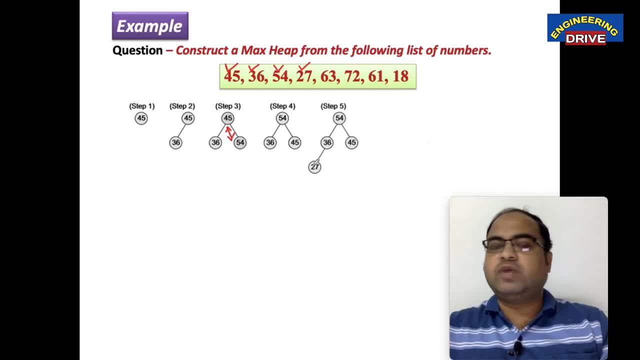 child of this: 36, 27. okay, now, whether it is following max hip property. yes, 36 is greater than 27, no problem. next insert 63. 63 inserted, but it is not following the max hip property because 36 is less than 63. that's why what we need to do, we need to swap them. 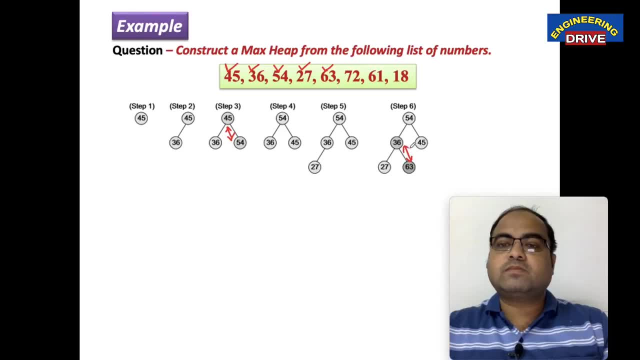 we need to swap them. okay, 63, 36, even this 54 is less than 63, even it is not following max hip property. so that's why we need to swap them. so what? we will get 63, 54. now, it is following the max hip property, no problem. then you start inserting the next element. so, dear students, 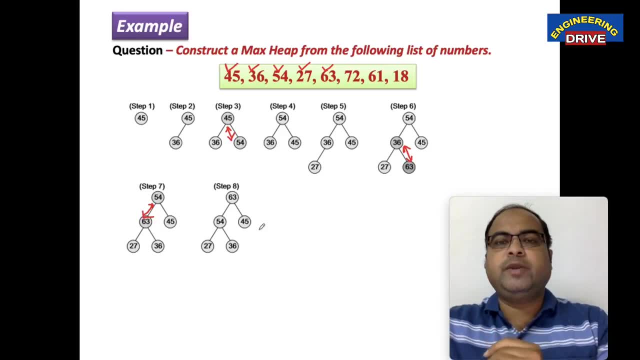 checking the condition of max hip property. so, dear students, checking the condition of max hip position. if it is following no problem, immediately insert the element. if it is not following the max hip property, then you need to heapify. we can call this procedure as heapifying the heap tree, or we. 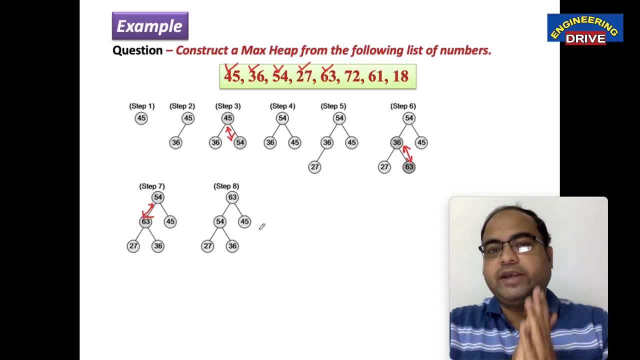 can call it as heapifying the binary tree. so we need to heapify it. okay, so 63. okay, next element: 72. so i will insert 72 now, so 45. the 72 will be stored as the left child of 45. node, is it clear? 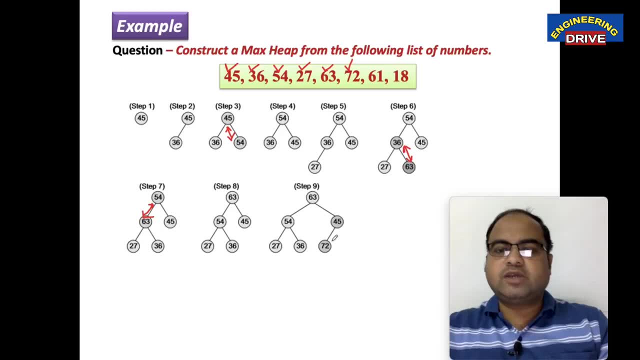 now, even this: it is not following the heap property, yes or no maxi property. so what we need to do? we need to swap, is it clear? so 72, 45. now tell me the next step, can you guess? yes, 63 is less than 72. even it is not following the maxi property. so just, we need to swap them. 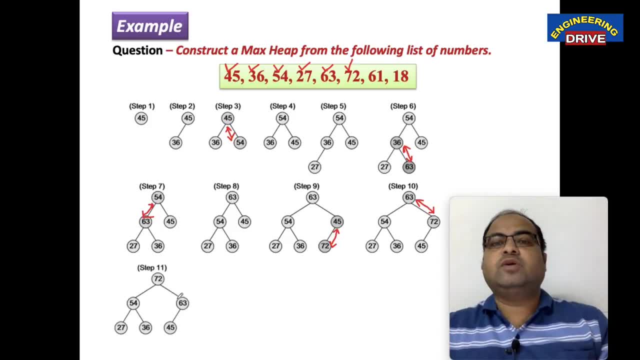 okay, now it is following the maxi property. clear. next step: we need to insert the next number, 61, where the 61 should be inserted. 61 should be inserted here: 61. okay, whether it is following maxi property. yes, it is following maxi property, there is no problem. then the last element we need to insert is what? 18.. tell me, can you guess? 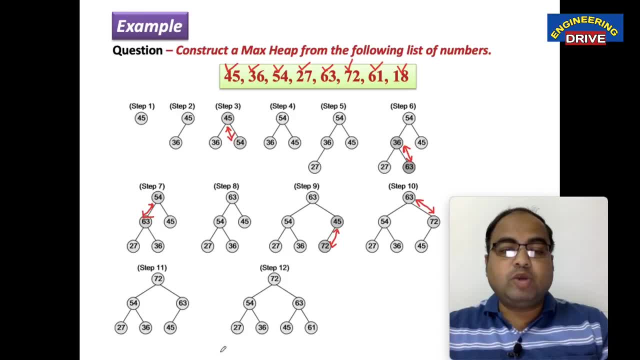 where the 18 should be inserted, whether it should be inserted below 27 as the left child or left child of 45. the answer is left child of 27.. so inserted successfully 18. so up to here, our algorithm closed, okay. so, dear student, this is. 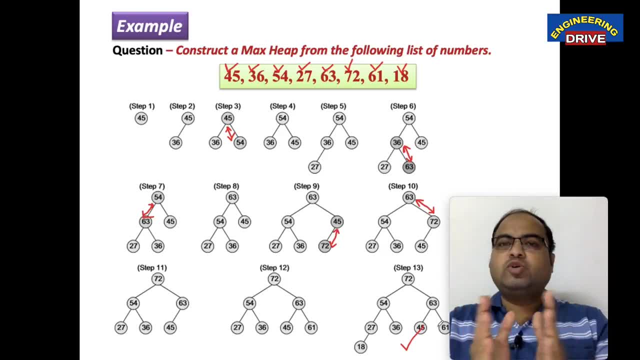 how we can generate a maxi now when we should know whether our answer is 100 correct or not. you should see the root node. it should contain the largest number in the array, in this unsorted array, it should contain the largest number, which is the largest number here. 72 is the largest number, so 72. 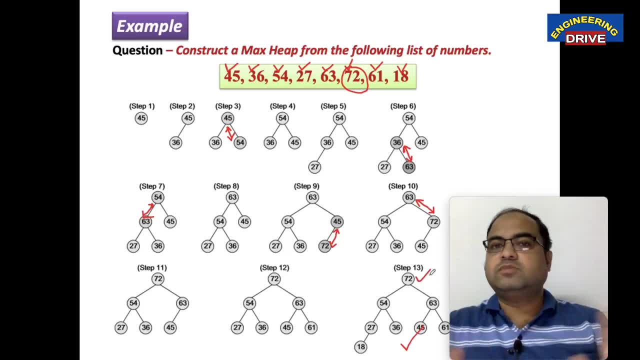 is available at the top. so maxi generated and the smallest number will come as the last value in the lowest level of the binary tree. so which is the smallest number in this entire unsorted array? 18. so we got 18 here. so our algorithm is 100 correct. so we have successfully generated a maxi. similarly, you. 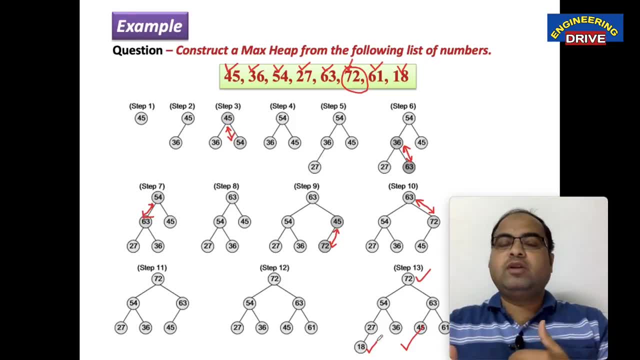 people. you can take it as the assignment and you can construct a minimum heap or min hip from the following same set of numbers. now you know what you will get from this set of numbers. you will get answer at the last. i will show you just, i will tell the random answer here you will get at the